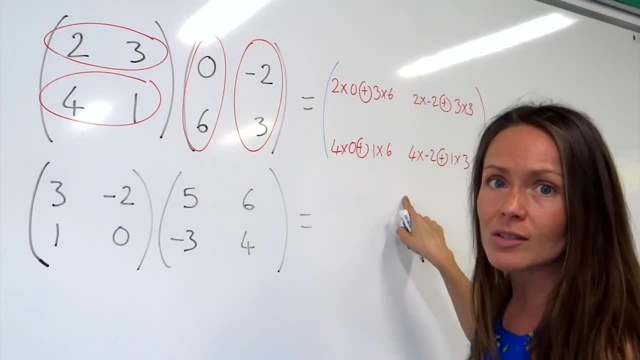 And you won't necessarily need to write them down. Okay, So I'm going to use the bottom row and the right column to find the bottom right element in the answer And I'm going to write down all of what I've just done here. 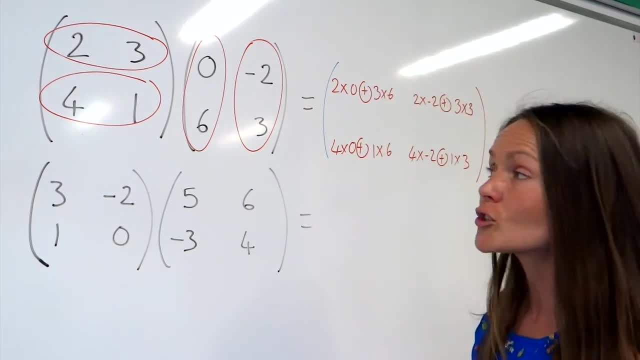 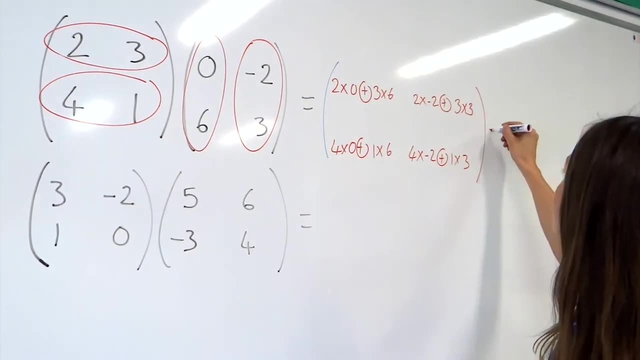 This is just to help you see the working out, to show you how I'm getting from here to here. So obviously we can't leave it like this. We've got to work it out now. So in the final answer, your 2 times 0 is just 0.. 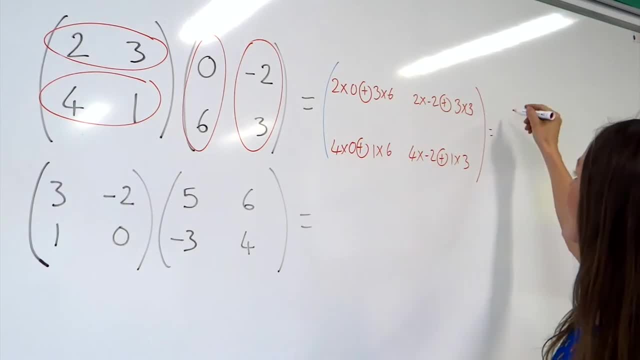 And 3 times 6 is 18.. So the top answer is 18.. For the top right I've got 2 multiplied by minus 2, which is minus 4.. And 3 times 3 is 9.. 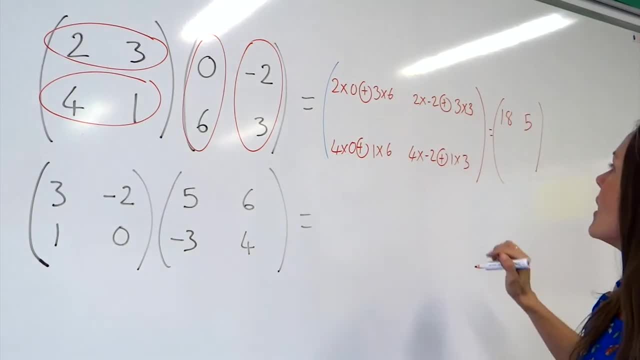 So minus 4 plus 9. Is 5.. Now for the bottom left. 4 times 0, again is just 0. And 1 times 6 is 6.. So 0 plus 6 is 6.. 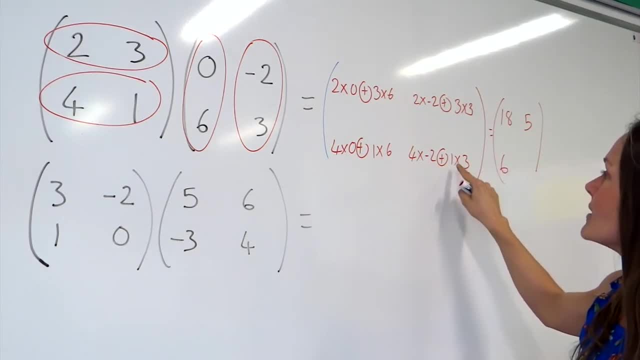 And for the last one, 4 times minus 2 is minus 8.. Plus 3 gives me minus 5.. So there's multiplying matrices. Okay, Now for the next example. same as before, I'm going to draw rows around the first one. 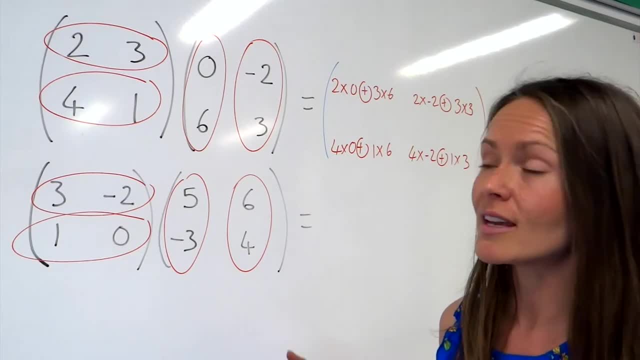 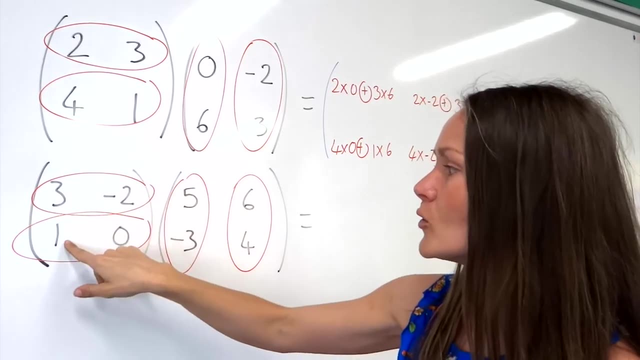 Columns around the second one. Okay, You don't have to do this, but I think it's useful so that when you're multiplying and adding, you don't stray out of that row and start using this one or this column and then start using this one. 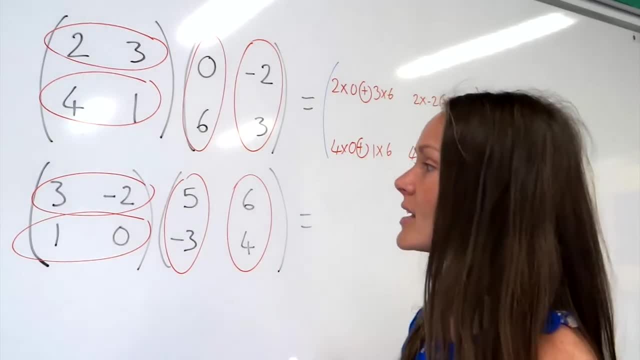 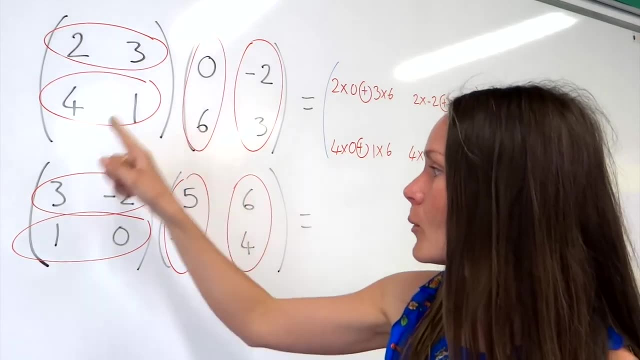 It's just as a guideline, But, like I said, you don't have to do that. It's just something that might help you when you're multiplying. So again, when you're multiplying 2 by 2 matrices, your answer will be a 2 by 2 matrix. 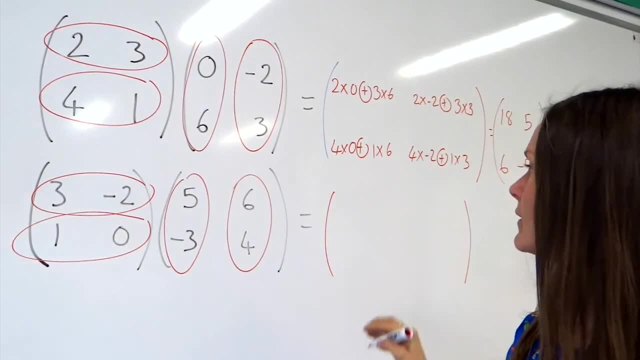 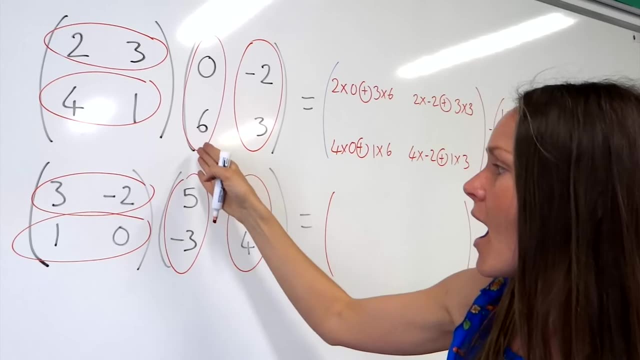 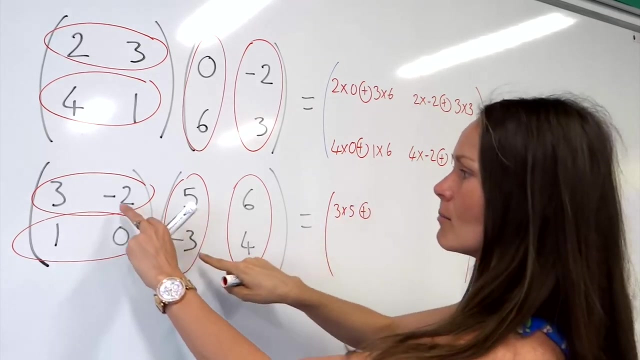 So I'm going to leave enough room for my working out here And to find the top left element in our matrix. we use the top row here and the left column here, So you're doing 3 times 5 plus minus 2 times minus 3.. 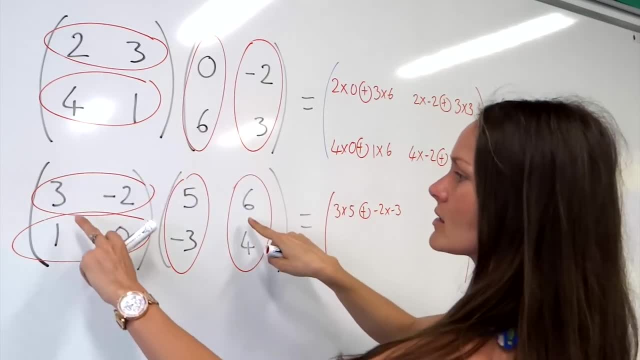 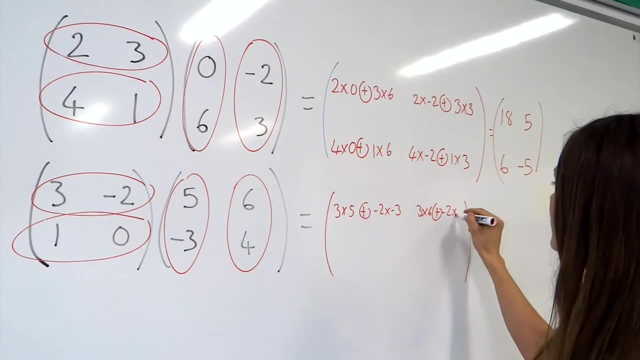 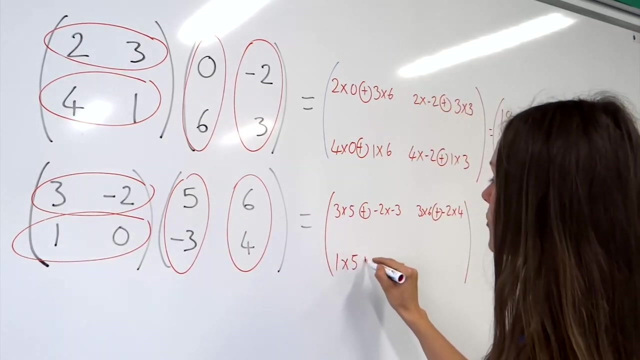 For the top right: use the top and the right. So 3 times 6 plus again minus 2 times 4.. Now for underneath, for the bottom left, use the bottom and the left 1 times 5 plus 0 times minus 3..